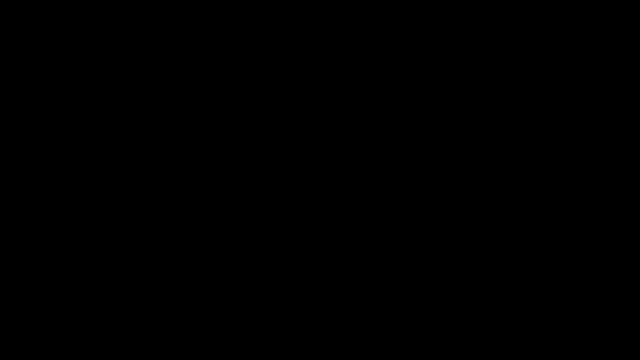 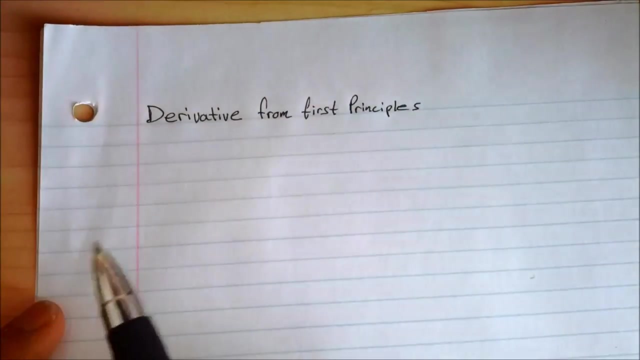 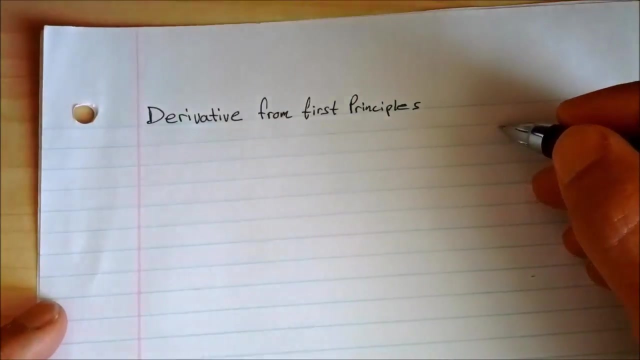 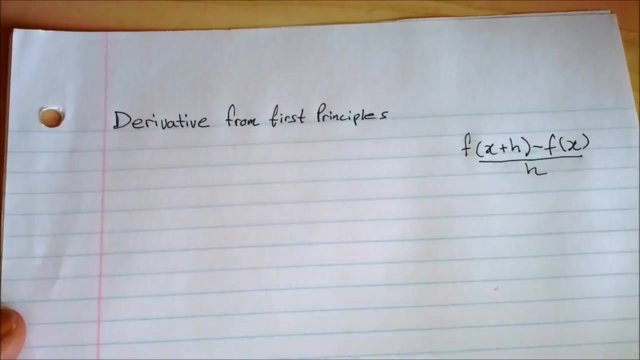 Okay, in this video we're going to find derivatives from first principles. There's one thing to keep in mind when finding the derivative from first principle, and that's if you remember this formula here. the rest is fairly simple, So I'm going to give a few examples and show you how to. 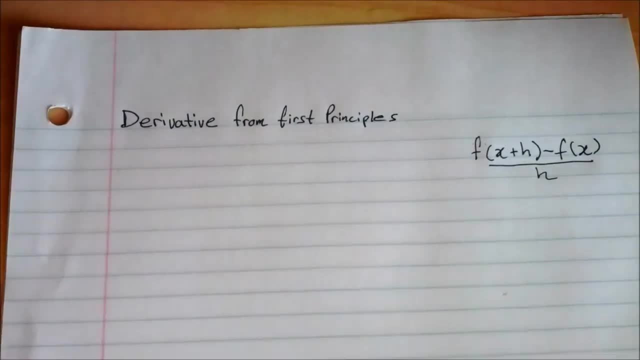 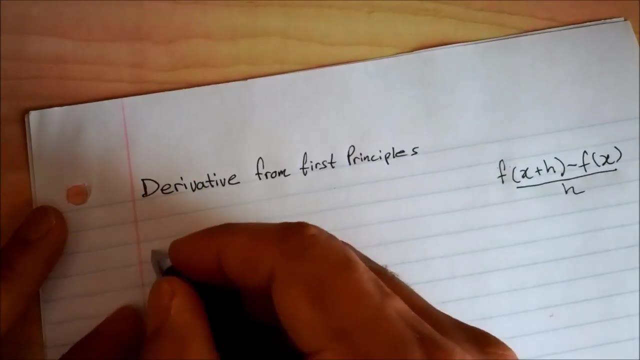 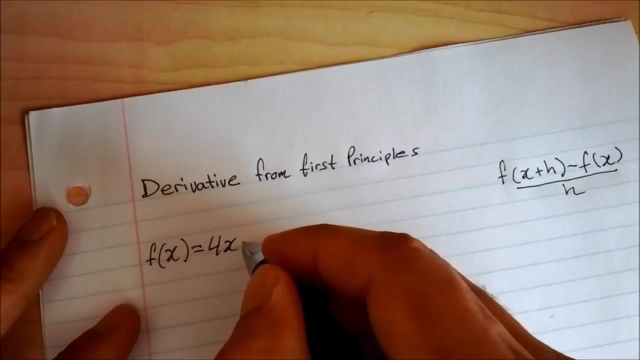 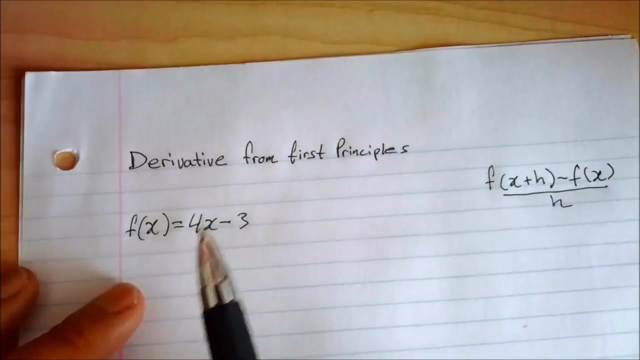 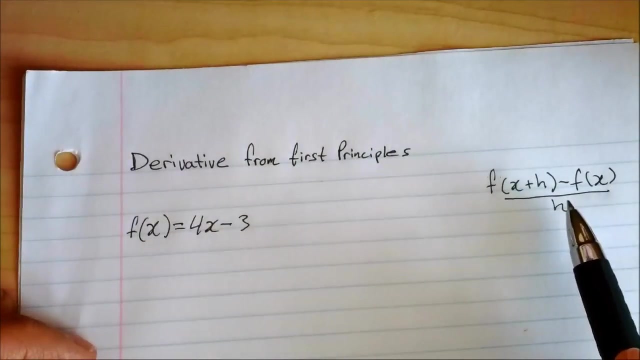 incorporate this formula into any given equation. Okay, here we go. so our first one is f of x, e minus b. f of y Equals 4x minus 3.. Okay, so what we do here. anytime you see an x in the function, you plug in this here. 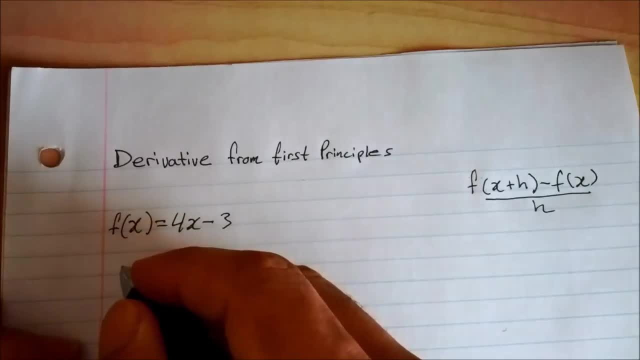 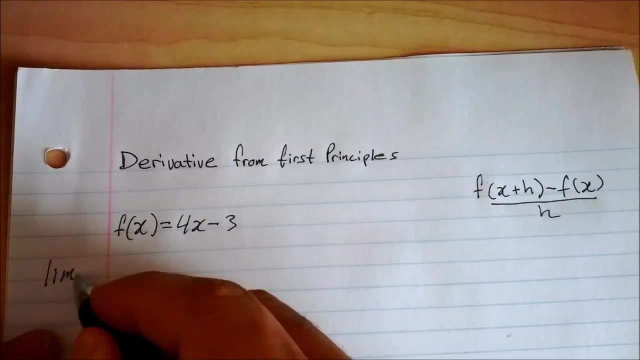 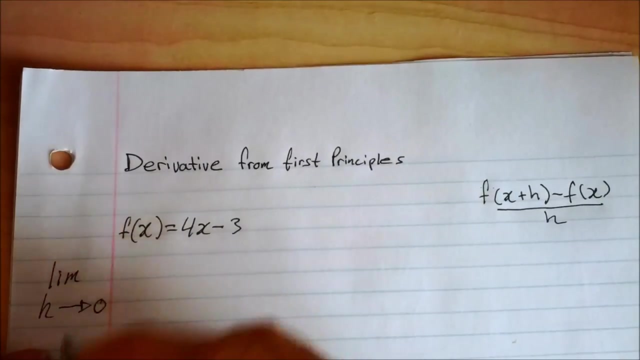 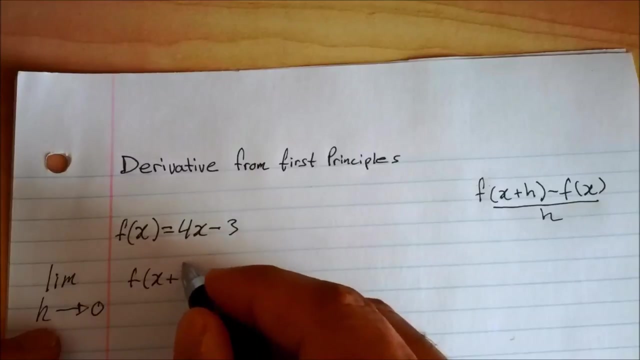 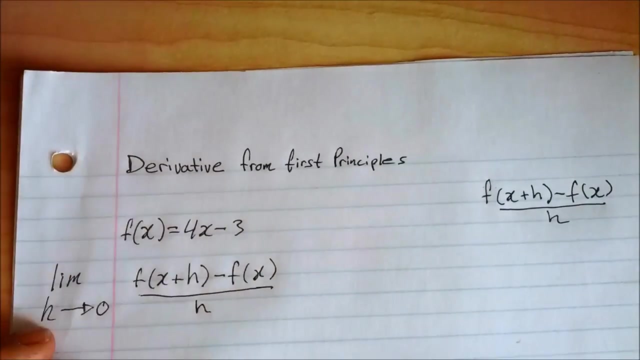 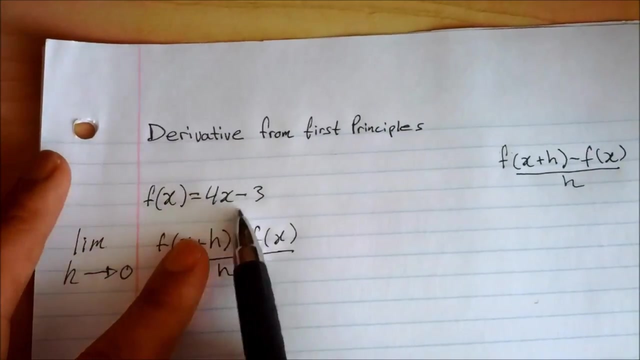 Okay, so here it goes, And of course, you're evaluating a limit- This is part of the whole process- And we use h, But as h approaches 0.. Okay, so this is how it is. Now we just plug in this value into this. 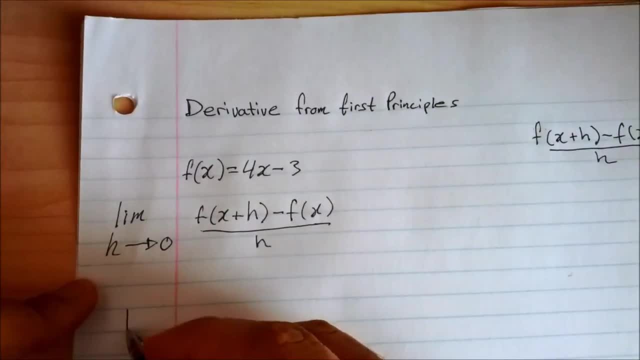 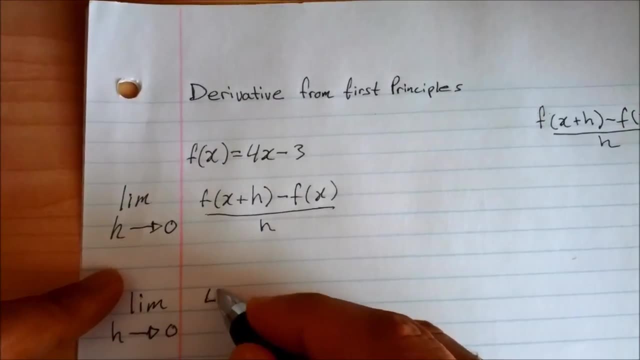 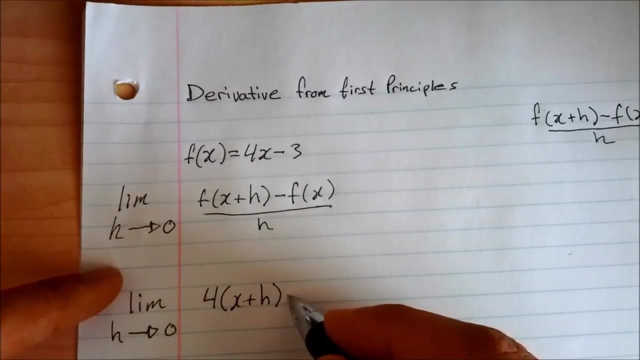 So what we do here: anytime you see an x in the function, you plug in this here. So what we do here: anytime you see an x in the function, you plug in this here. So what we have here is limit as h approaches 0 for x plus h minus 3.. 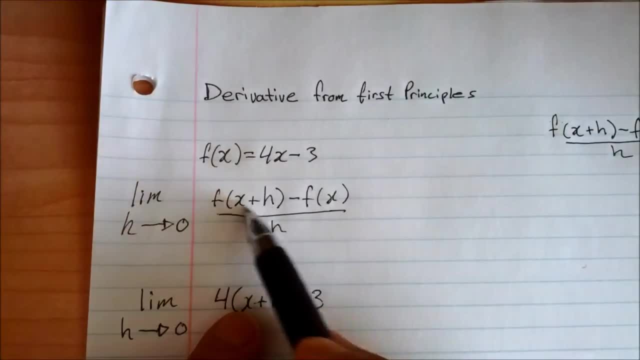 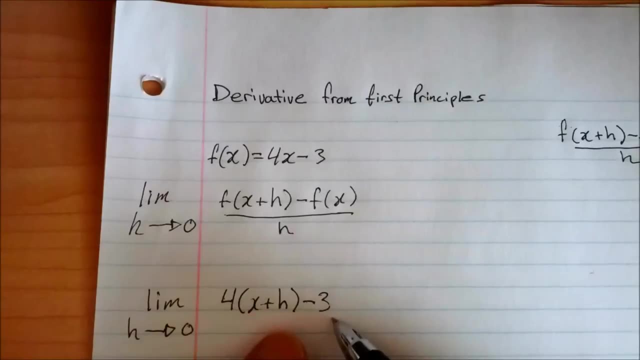 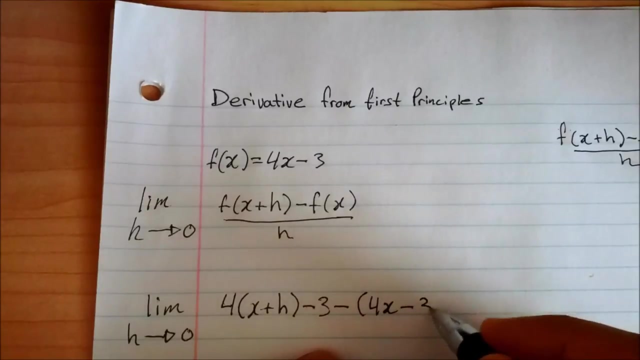 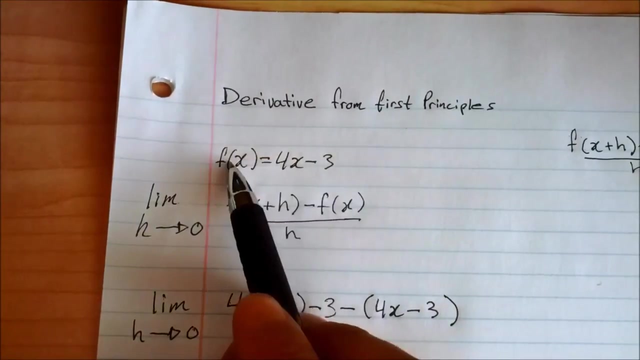 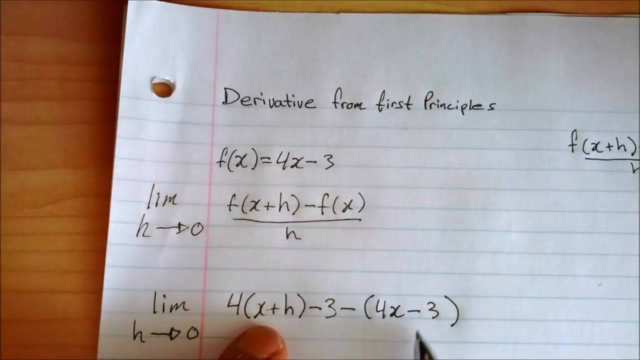 So where we saw this x, we plug this in And it's take away the original function. So take away 4x minus 3.. So we plug in the x plus h into any x value in the function And it's take away the original function, which is here. 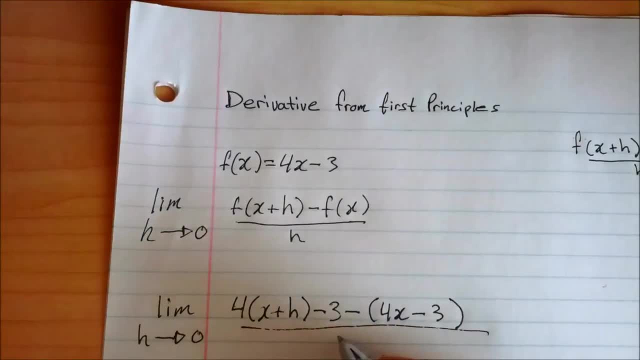 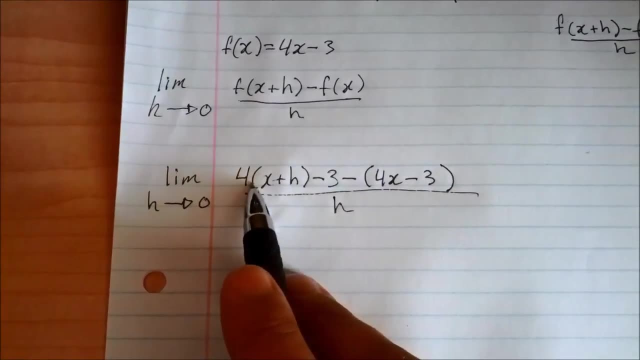 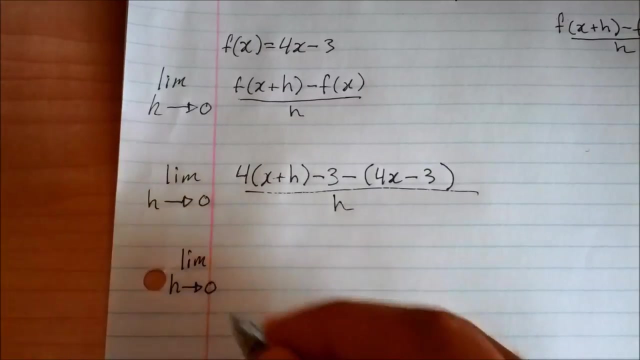 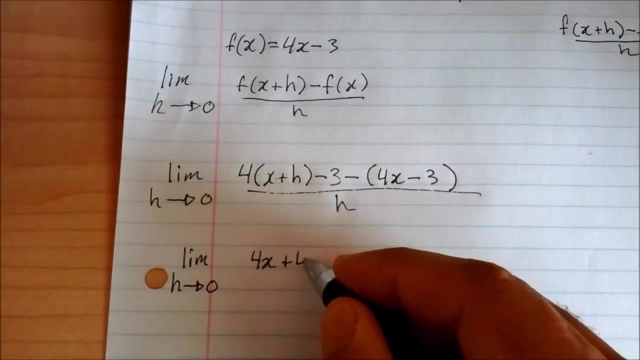 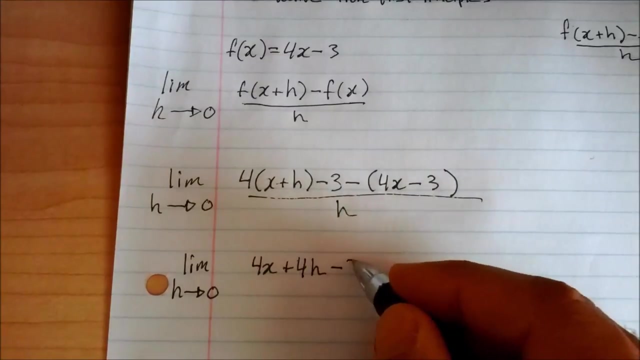 And it's all over h. Okay, so we go ahead and you know, work this out. So, as limit h approaches, 0, 4 times x is 4x. 4 times h is 4h. Okay, so negative 3 here, of course. 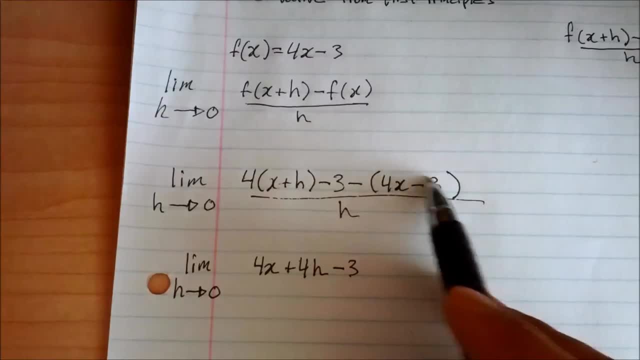 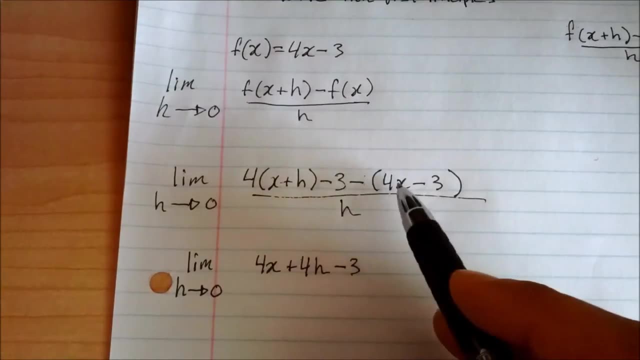 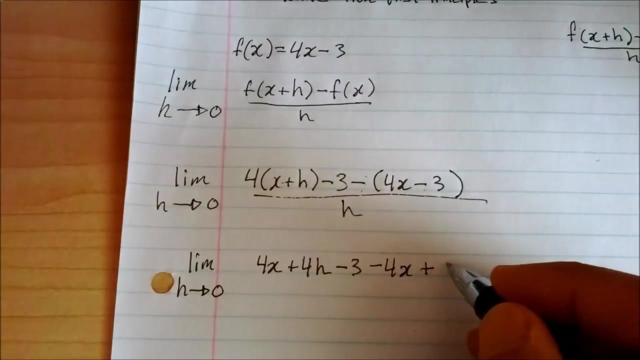 We keep the negative on the outside and put the original function in there. We keep the original function in the brackets to make it easier to multiply. So negative times 4x is negative 4x. Negative times negative 3x gives us positive 3.. 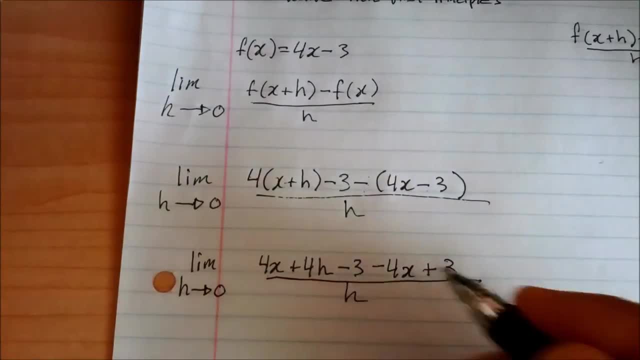 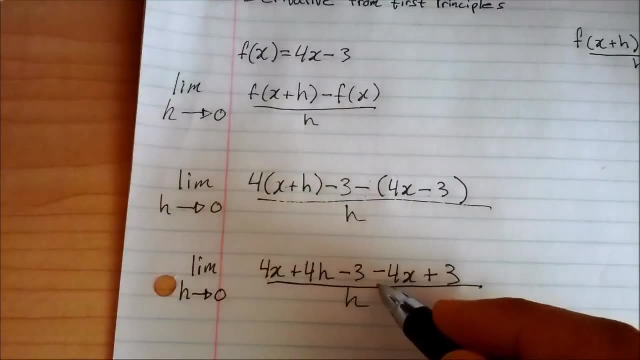 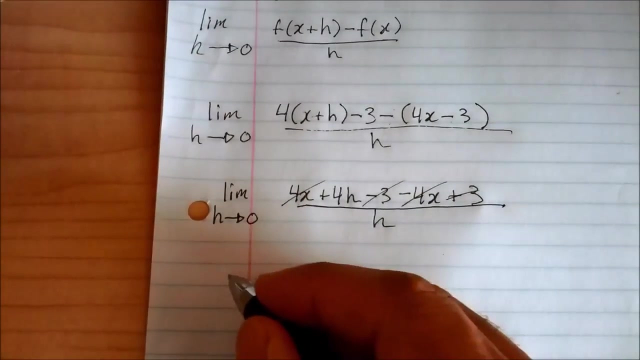 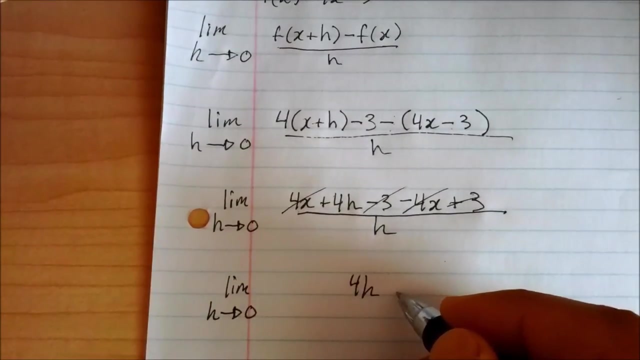 Okay, and that's all over h, So we can go ahead and cross terms out, cancel out terms here. So negative 4x, 4x. Positive 3, negative 3.. So as limit h approaches 0, we're left with 4h over h. 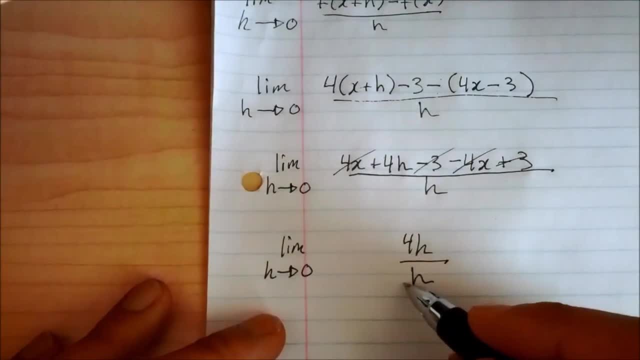 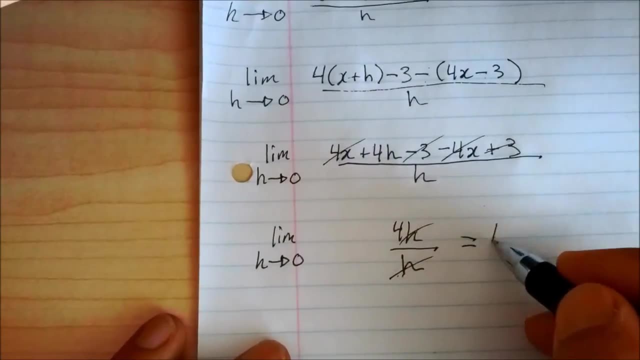 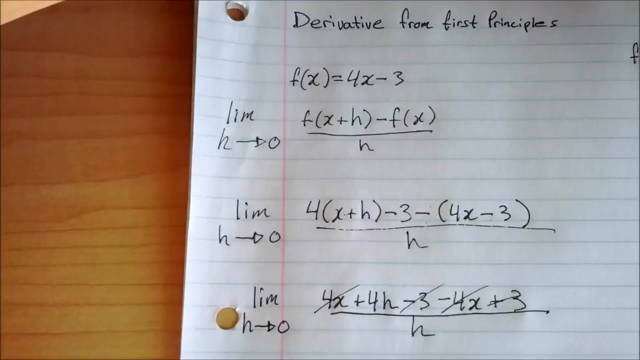 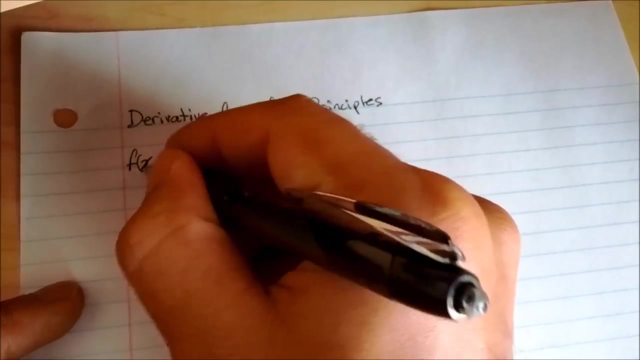 Okay, and right now, of course, they're dividing. You can cancel them out And you're left with 4.. We're left with 4.. Okay, in this example we're going to do: f of x equals x squared plus 4x. 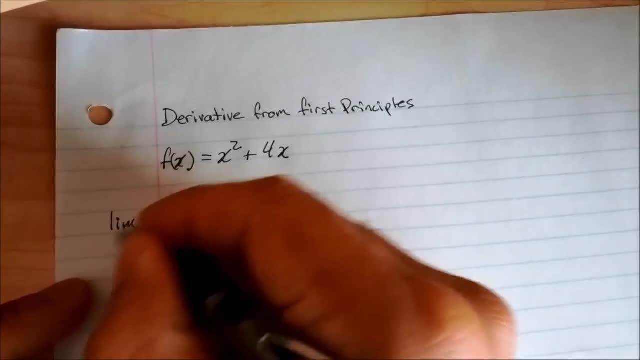 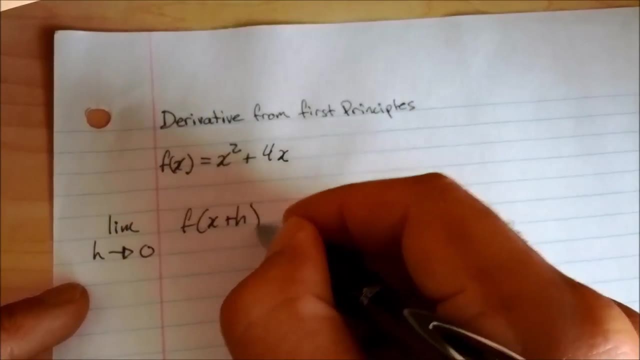 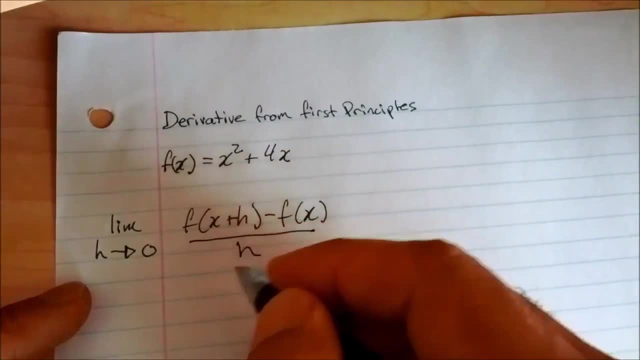 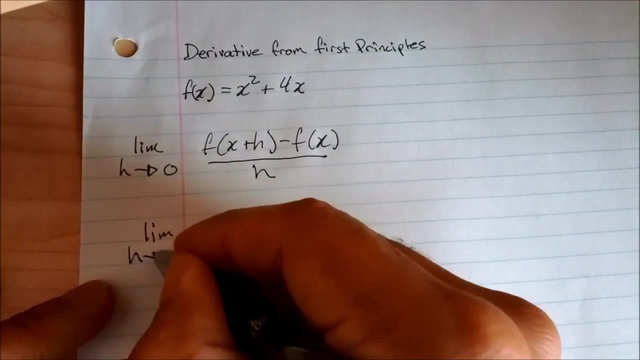 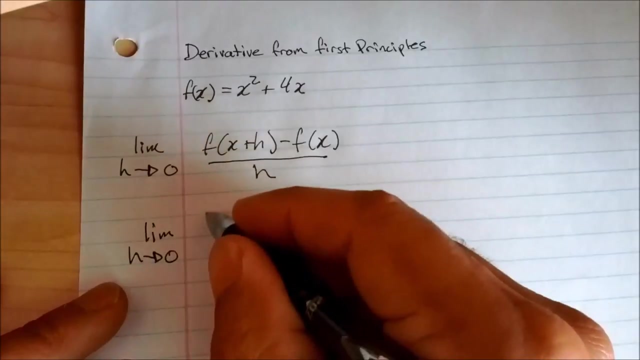 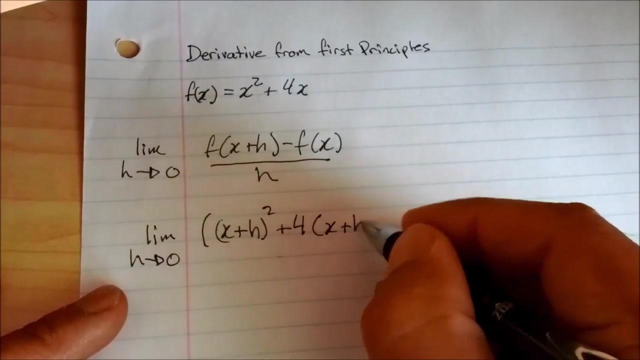 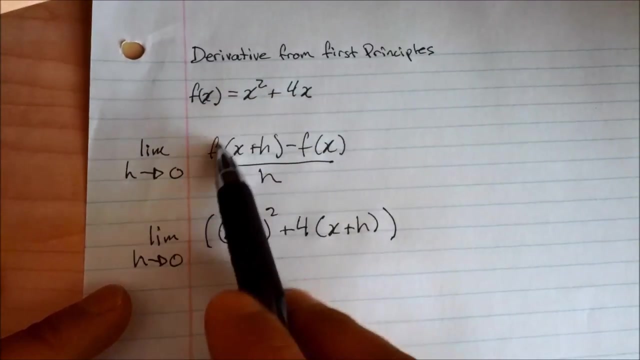 Okay, so Okay, there's our formula. So here we go. As limit h approaches, zero, x plus h, squared plus four x plus h. So anywhere you see an x in the original function, of course you plug in x plus h. 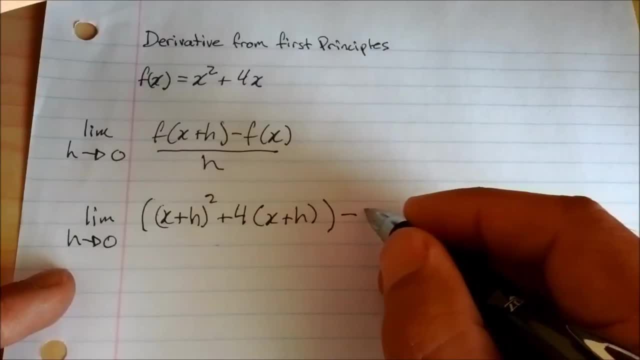 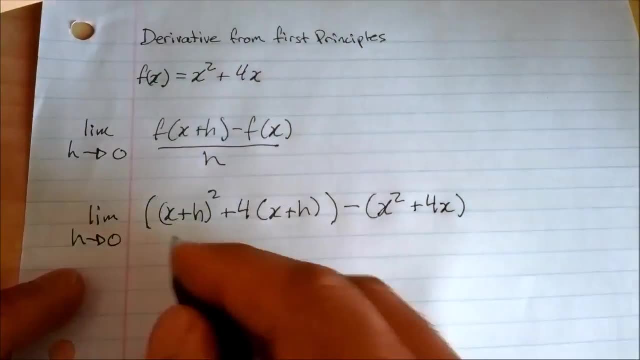 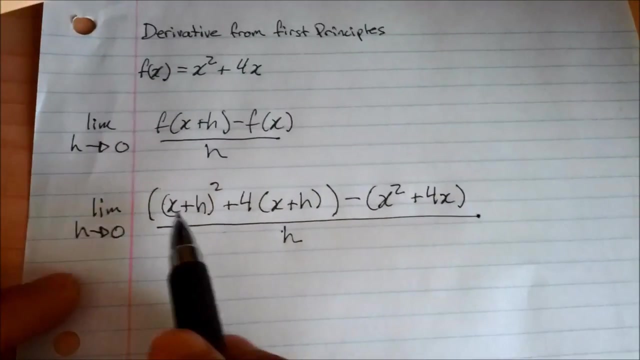 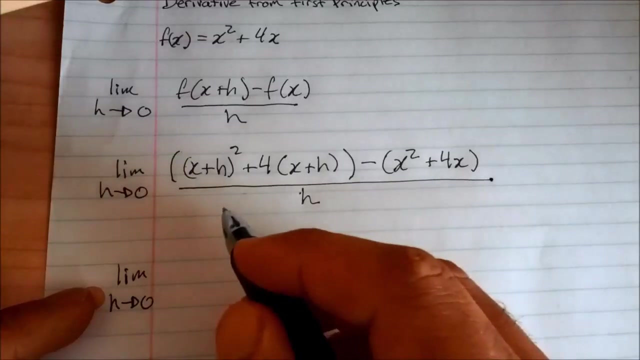 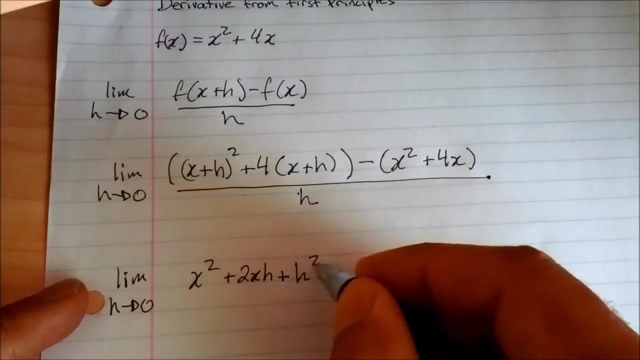 And that's all minus the original function. X squared plus four x And that's over h. Okay, and right here we can just expand these brackets. Okay, So x plus h squared is always x squared plus two x. h plus h squared. 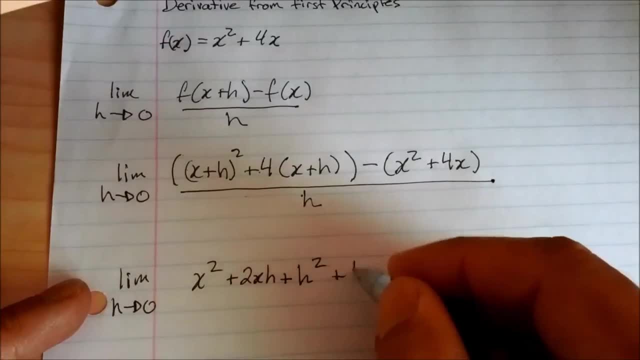 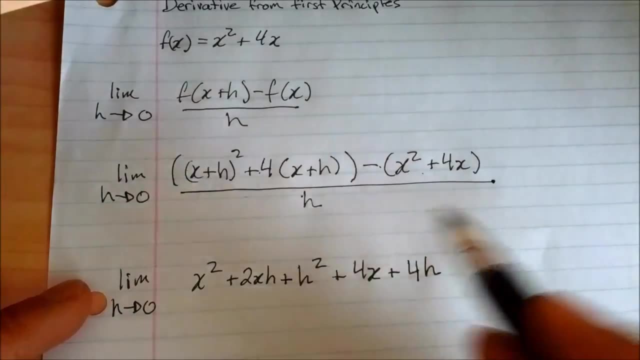 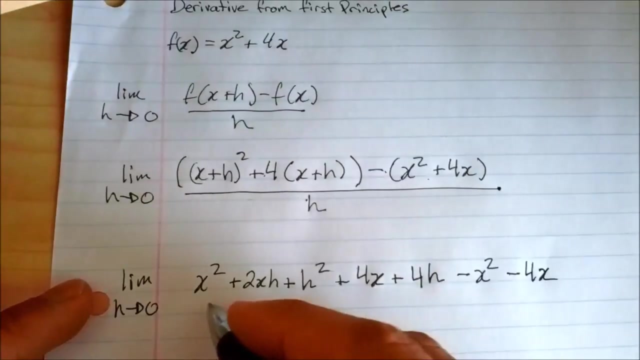 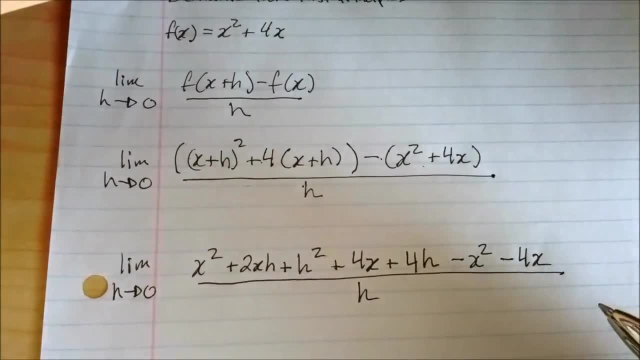 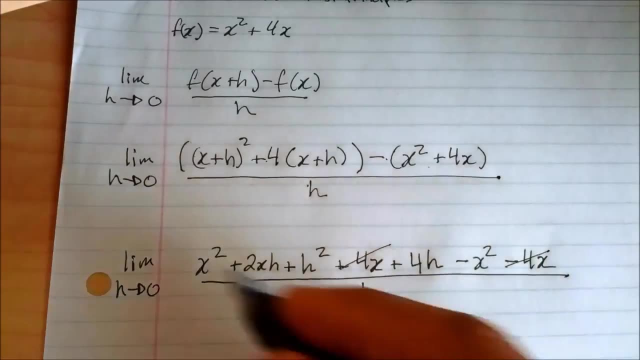 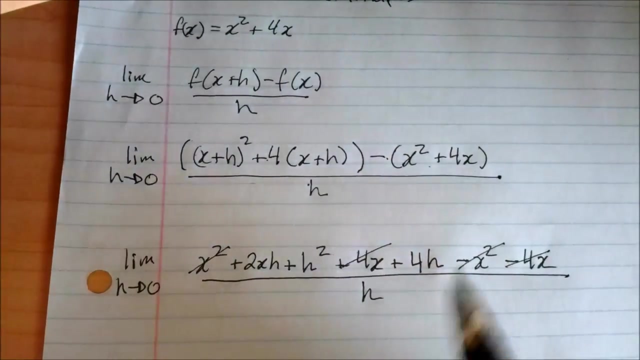 Negative four x And that's over h. At this point you can start canceling out terms and dividing. Okay. so positive four x, negative four x and positive x squared, negative x squared. Okay, and we have a few h terms that we can get rid of with this, using this h here. 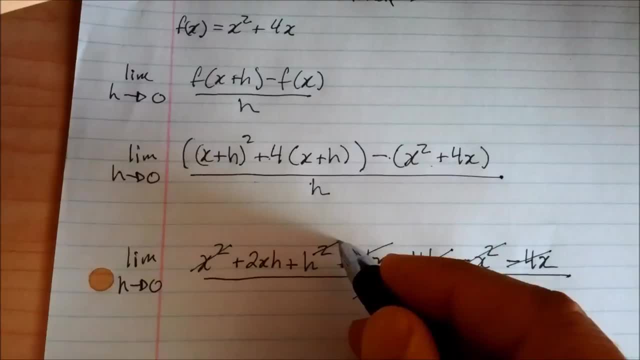 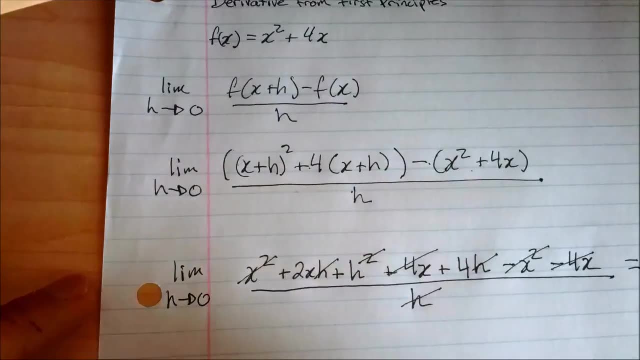 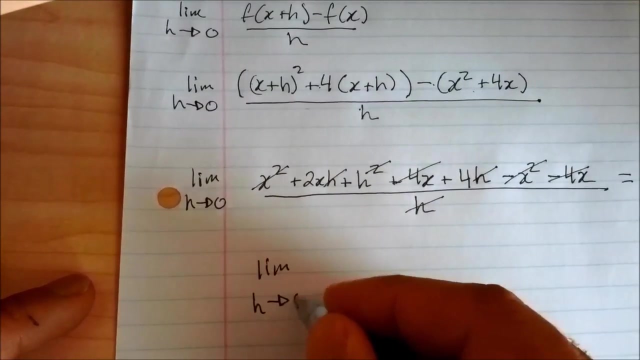 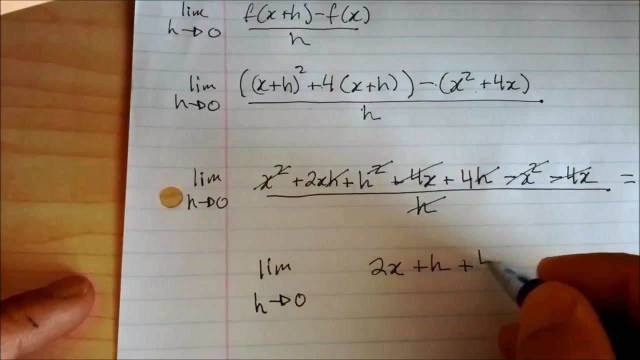 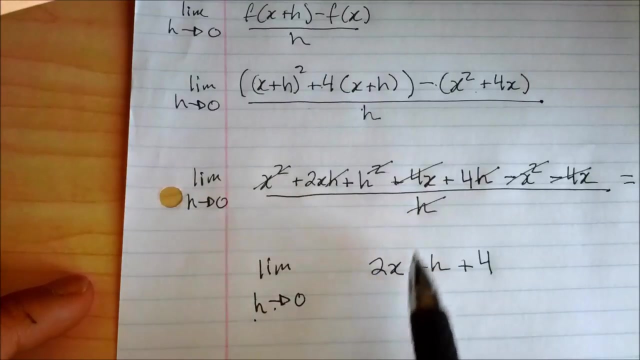 Divide this, Remove that, Remove one h, Remove this h also. Okay, Once you get rid of these h's, you're left with as limit, as h approaches zero, Two x plus h plus four. Okay, at this point you apply the h, you apply the limit, which is zero, and any instance. 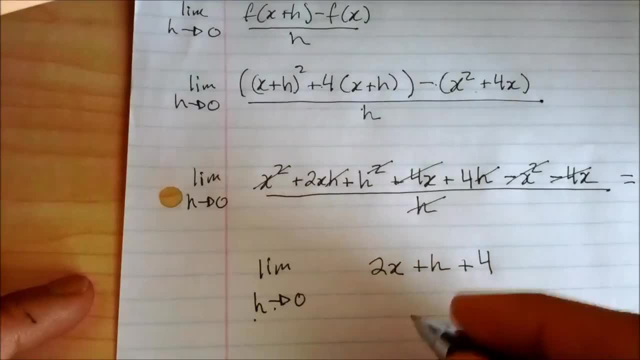 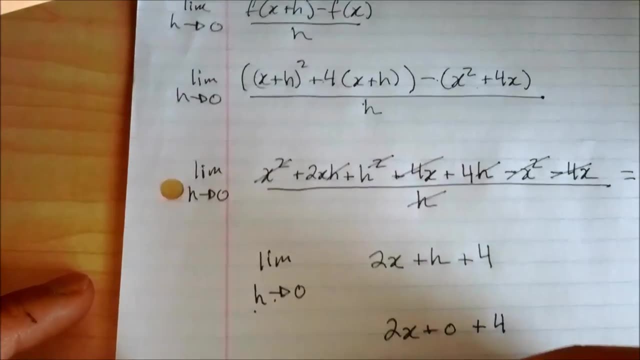 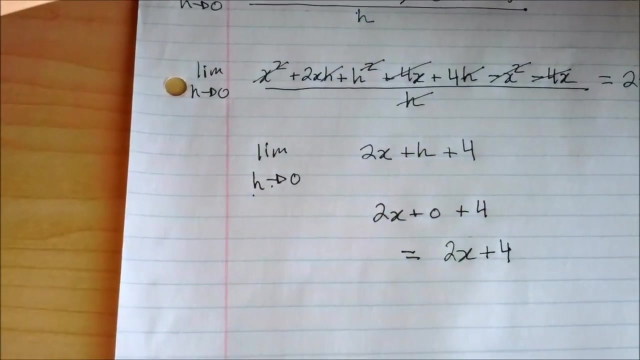 of h you encounter, you put a zero in, Okay. So two x plus zero plus four equals two x plus four, And that's it.